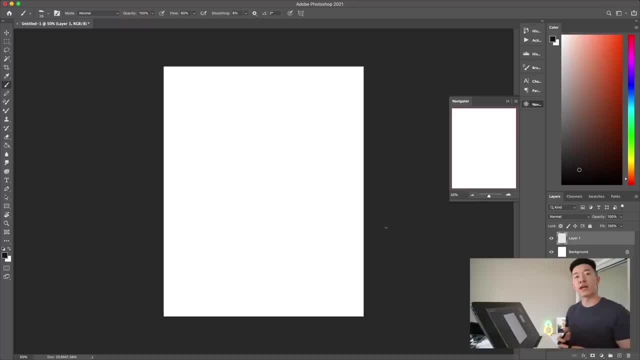 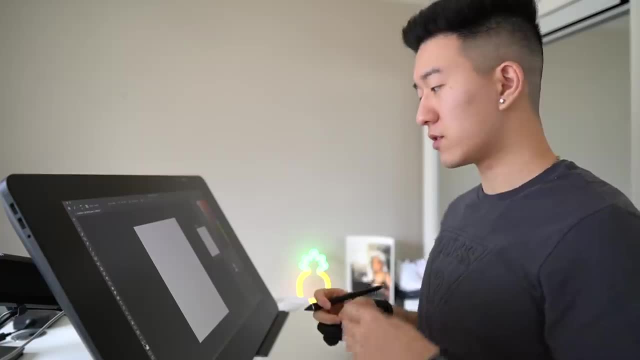 on. So I'm going to show you guys how to do this by doing a quick grayscale portrait, and then, throughout this process, I'll tell you guys a little bit more about why you should be doing this and some of the things that it can help you achieve. So let's get started. 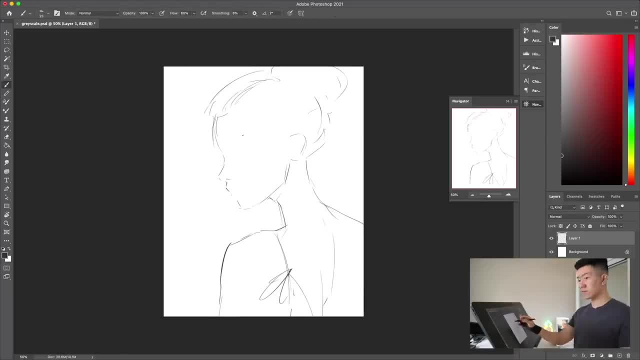 Alright. so now that I've gotten the sketch down, I can start getting into the rendering process a little bit. and the rendering is going to be very simple. We're just moving from the top of the slider down to the bottom of the slider. We're not worrying at all about the 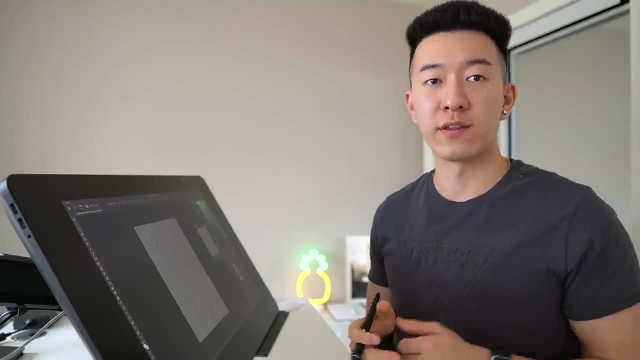 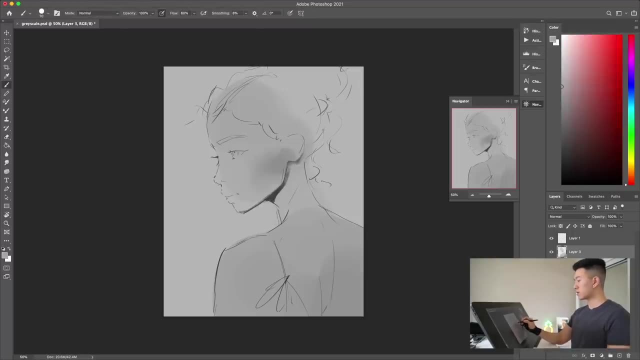 hue or the saturation, so you can really really focus on just one single thing. So this process is very similar to just sketching with graphite on paper, except we're doing this digitally. so it's going to save us a lot of time and it's going to save us some trees. 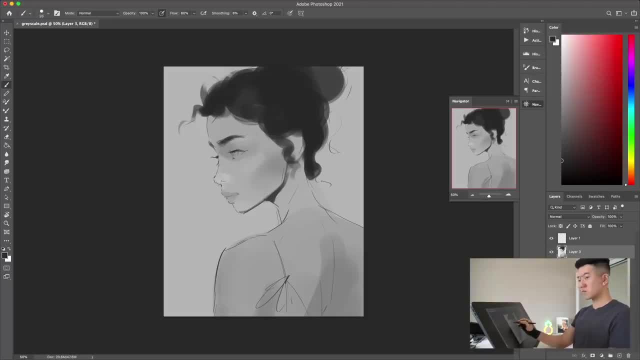 Okay, so you see that was very quick. That was about five minutes and we got a basic sense of the values down Now. the reason that was so quick is because we are just focused exclusively on the values and if you're somebody who, if you're rendering out an illustration, you find that 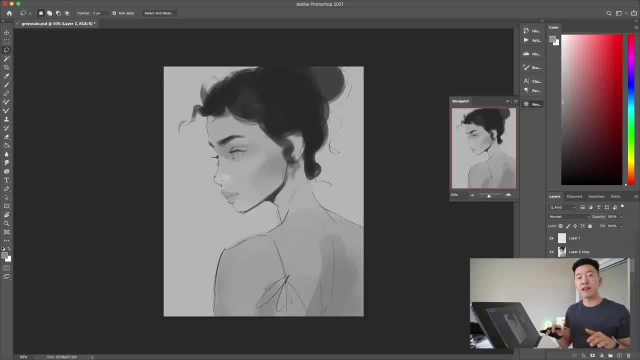 your colors or your lighting is looking a little bit flat as opposed to three-dimensional. this is something that's going to really, really help you guys, because you want to have a good understanding of values before you start approaching the values. So let's get started. So let's get started, So let's. 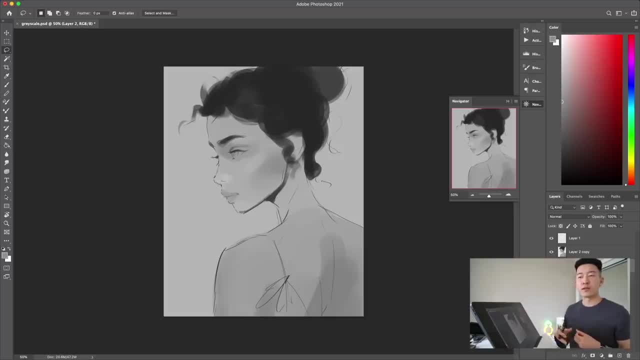 all the different colors, because the thing with digital art and art in general is just that you want to take things one step at a time. You want to learn one thing at a time. You don't want to get yourself way too overwhelmed with all the knowledge that there is about all these different. 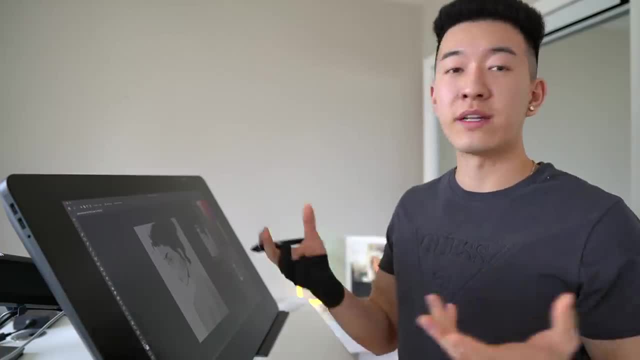 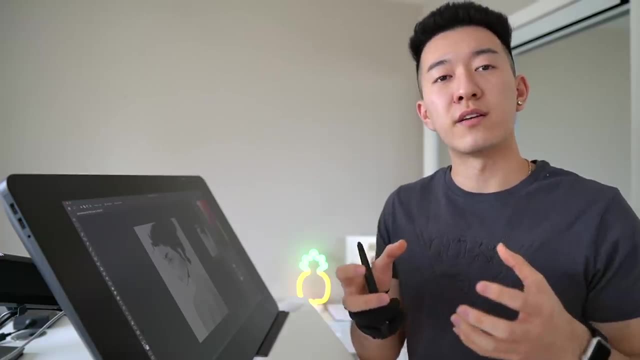 topics, Like if you're jumping into art fresh without any knowledge. there's so many different things. There's perspective, there's anatomy, there's color theory, there's lighting, there's all of these things that all come together to make you a good artist, So you have to really 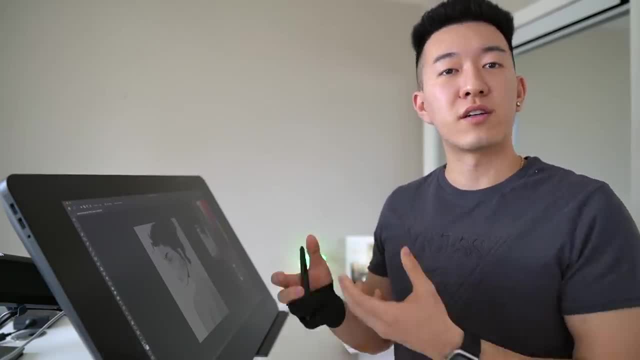 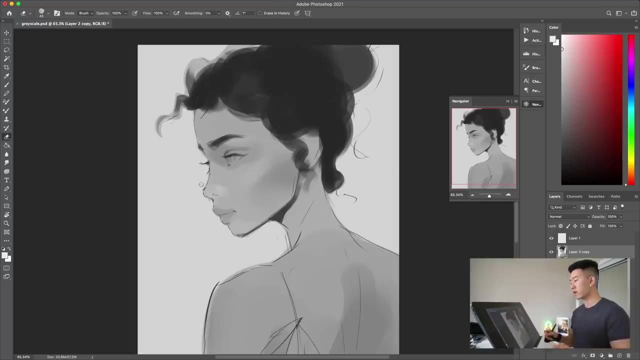 take things one step at a time. If you overwhelm yourself, chances are you're not going to be too happy with your work and you're going to have a hard time learning what it is that you need to learn. So now let's go back into this piece and flesh it out a 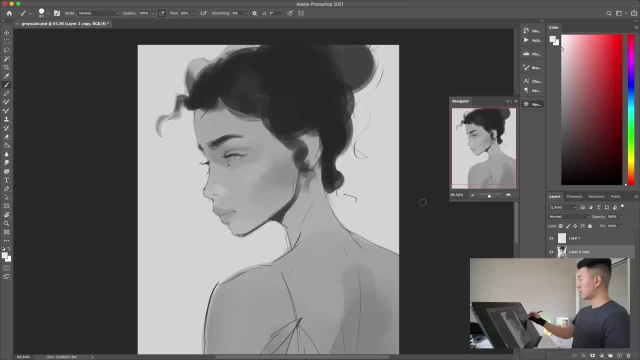 little bit, and this is just a very, very calming and satisfying process because you're not worried about the colors at all. You know, you can just kind of turn your brain off and only focus on the values that you see in the in the reference image. 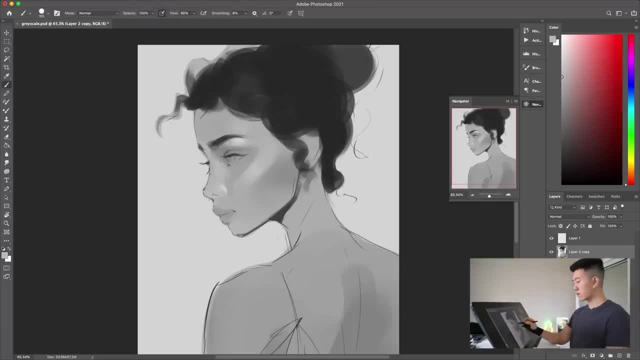 So the reason that I thought this video was important to make is because I was seeing people struggling with applying colors onto their illustrations, and where a lot of people have the most trouble is understanding where to push the darks and where to really pull the lights, and 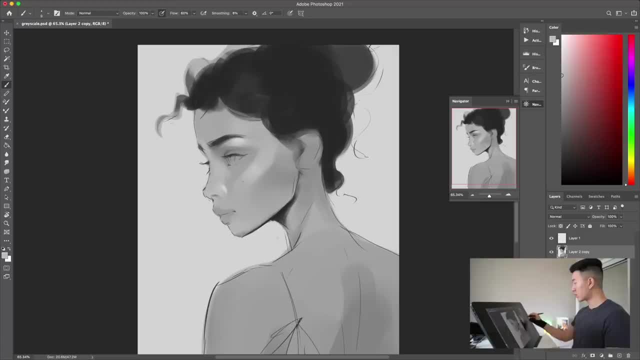 sometimes you know if you're drawing something and you're not sure what to do with it, you're not something. without good knowledge of values and how values transition into one another, your drawings might end up looking flat as opposed to three-dimensional. I mean like really understanding. 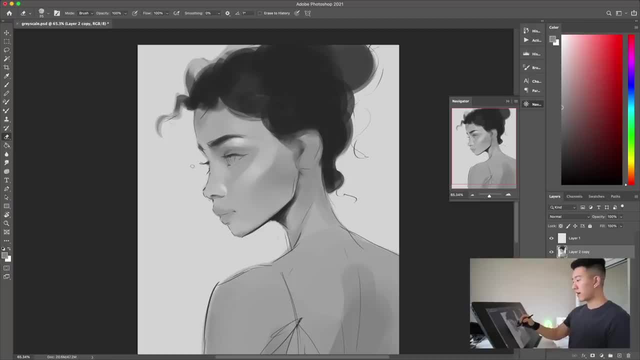 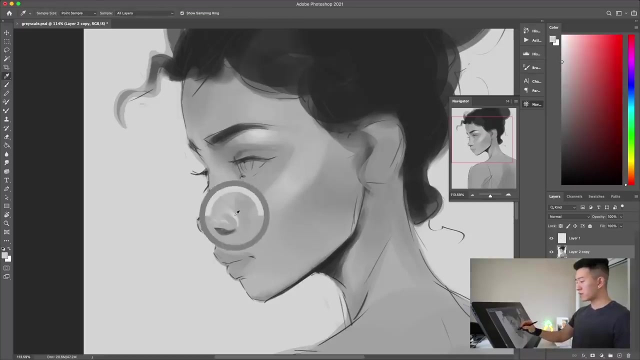 values is such a key component in any drawing. You know it doesn't matter if you're painting with or without colors. values are essential to any painting that you make. Now we're getting into the details a little bit, but you can still see everything in the drawing. 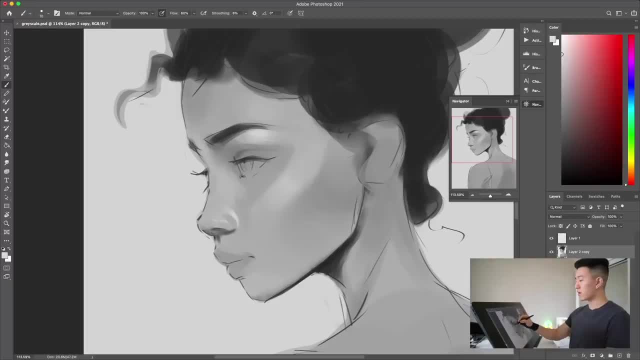 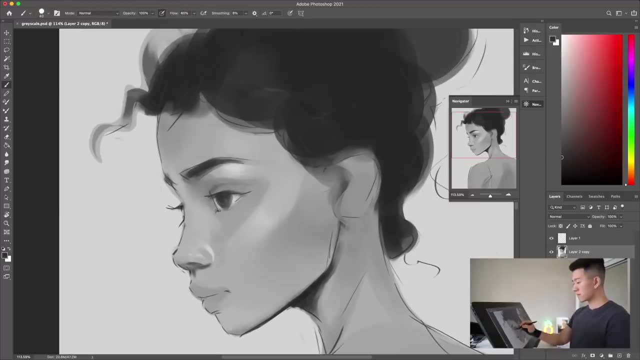 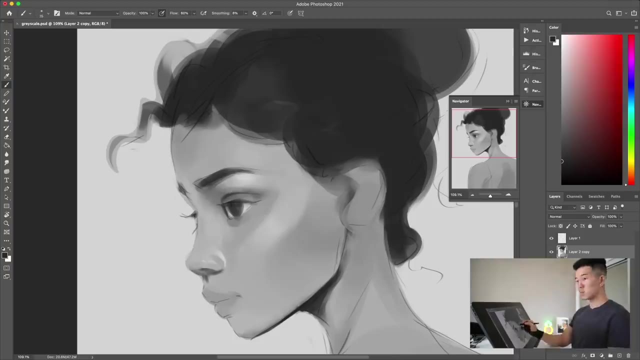 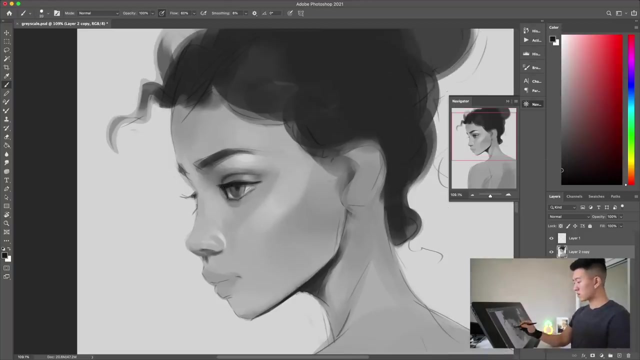 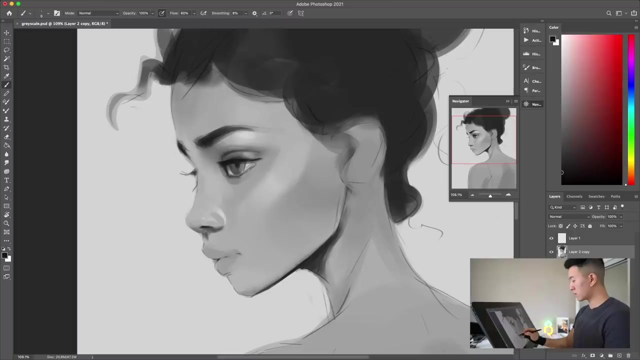 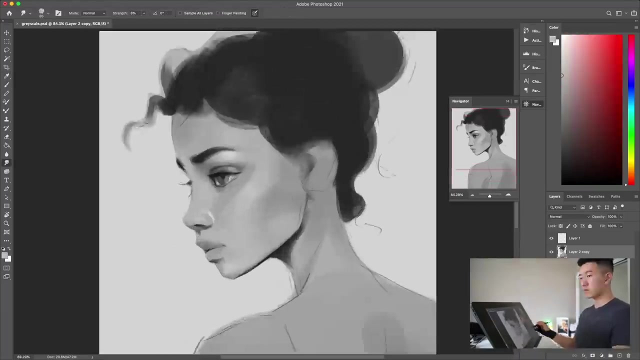 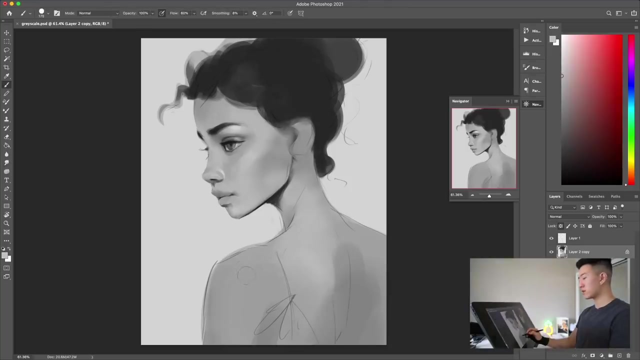 It becomes readable based on the values that you actually choose for each part of the painting. You can say a lot with values, and values only, Even if you think you are an intermediate artist. it never hurts to go back and brush up on your values once in a while, and you know what the good thing is about this, and you don't have to. 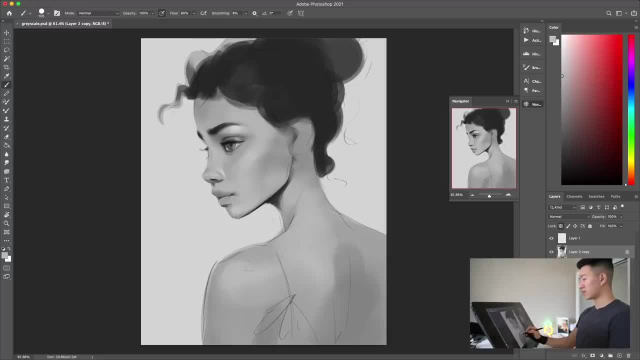 have a digital art tablet to be able to do this. You can just as easily do this with a pencil and paper. It might just take a little bit longer, but it's the exact same process and that's actually how I started learning how to draw. 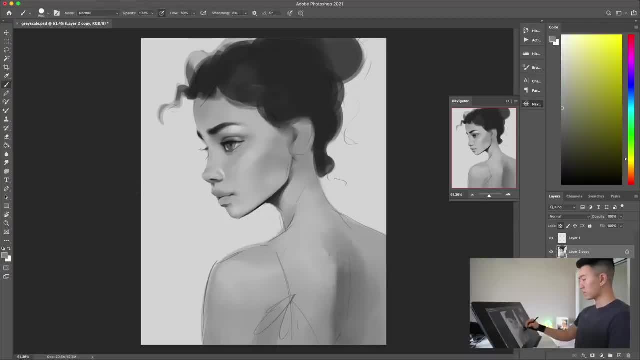 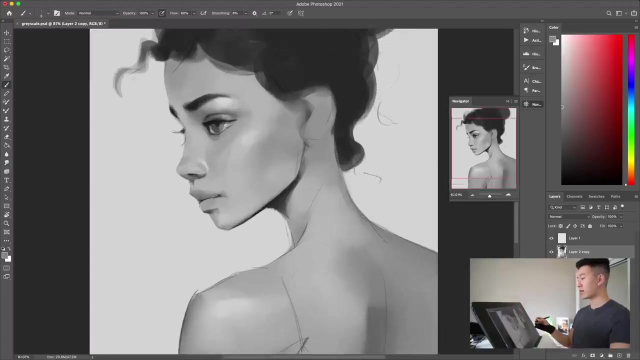 Sightly Music, Music, Music, Music. try this method and you happen to find it very difficult, more so than painting with colors. then that probably means there's a bit of a hole in your knowledge with values and you definitely want to patch that up. I really think that being able to paint and draw in black and white is one 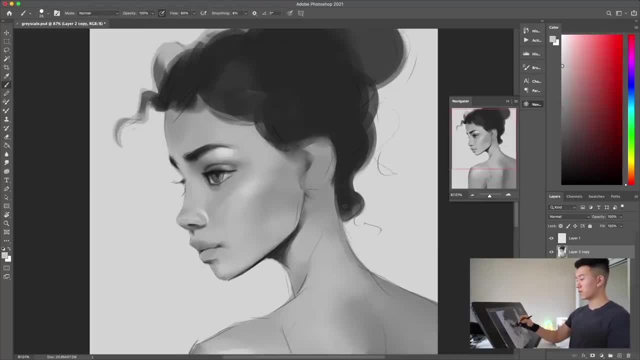 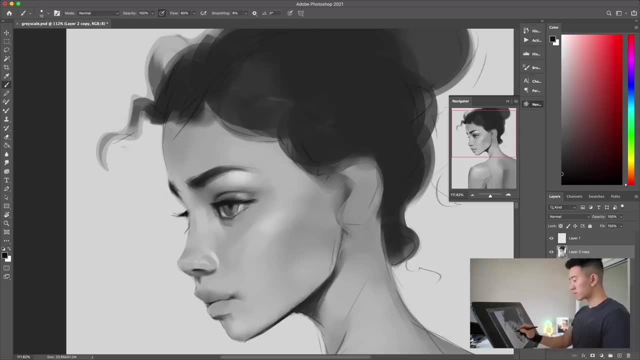 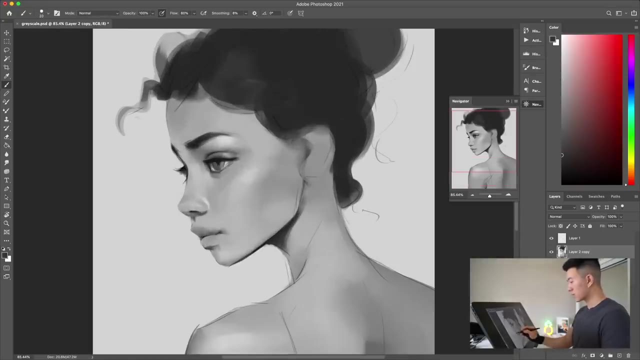 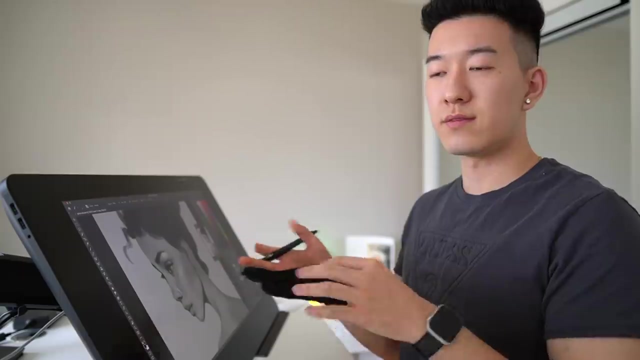 of the first foundational steps. It's one of the most important steps to becoming an effective artist. Also, when you're trying to do this kind of thing, especially on digital, try to avoid pure blacks- and I would say this goes for even you know- colored paintings as well. just like, always, try to avoid. 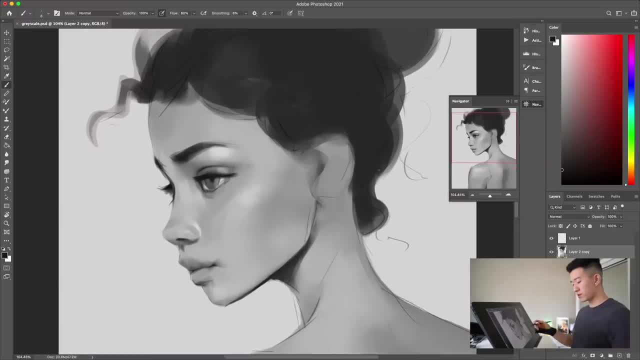 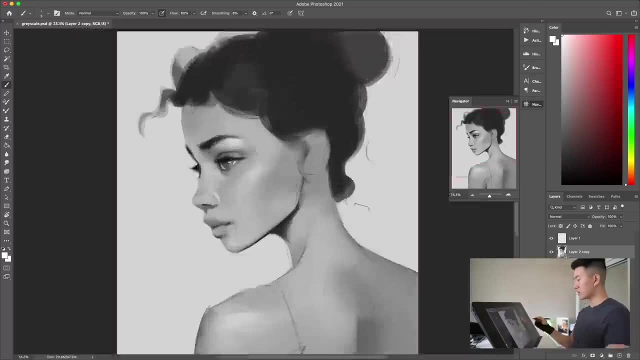 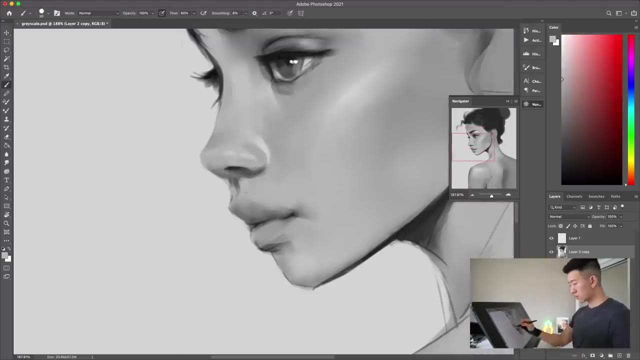 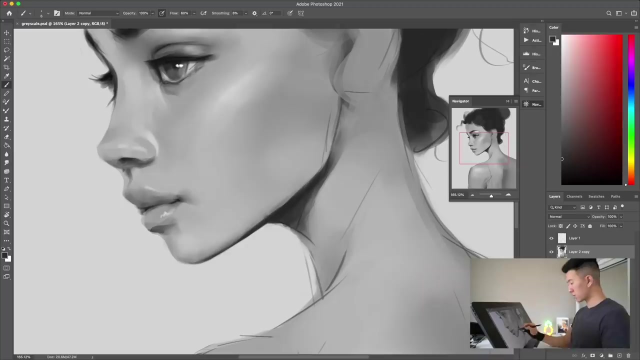 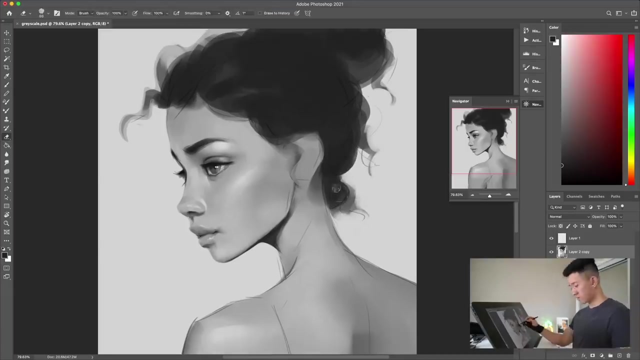 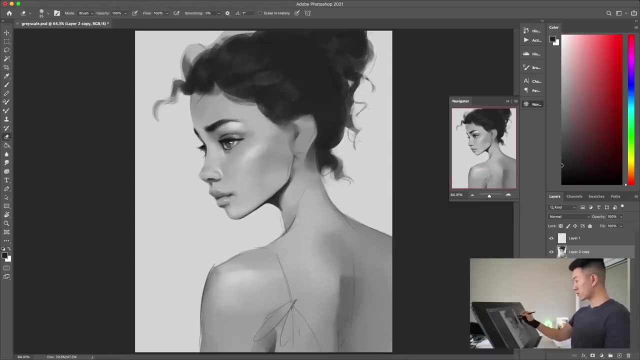 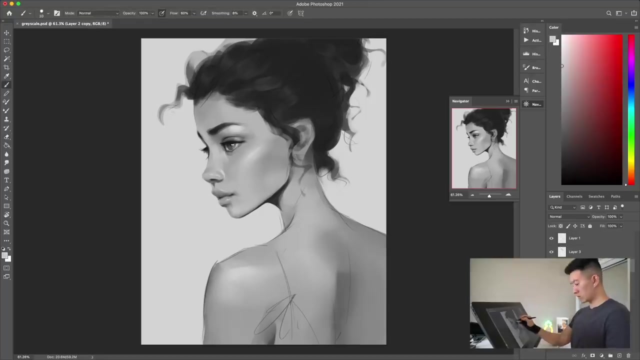 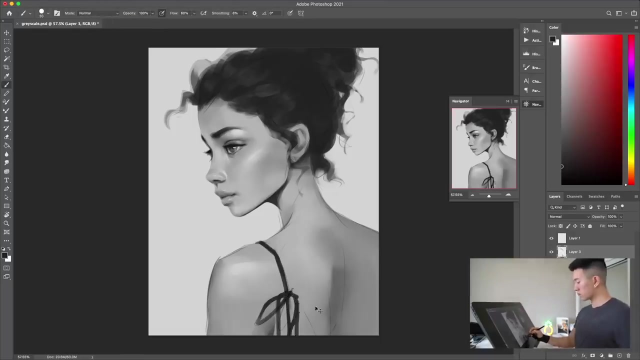 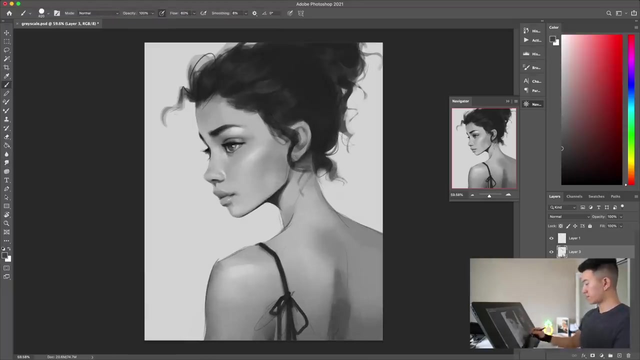 going down all the way to the bottom of the darkest possible color, because, especially on digital, it just seems very jarring when you go super, super dark. Thank you for watching. I'll see you next time. Okay, there we go. it's been about 15 minutes. here's the finished product. that was very, very fast and 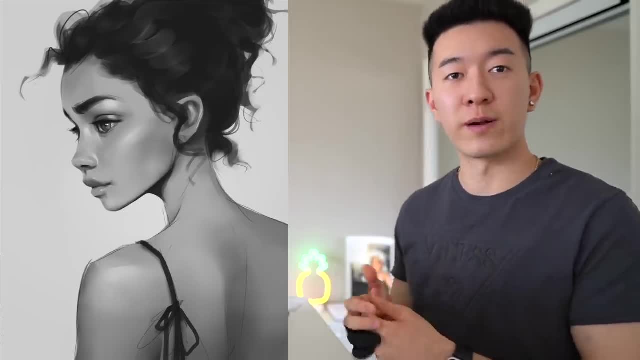 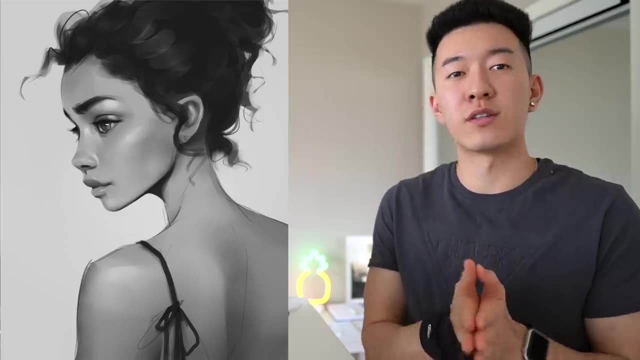 this was a really, really fun process to go through again and I think you know, if you are a beginner- again, like I said throughout this video, if you're a beginner and you don't really know where to start and you're having trouble rendering out your paintings and things are looking flat, this is 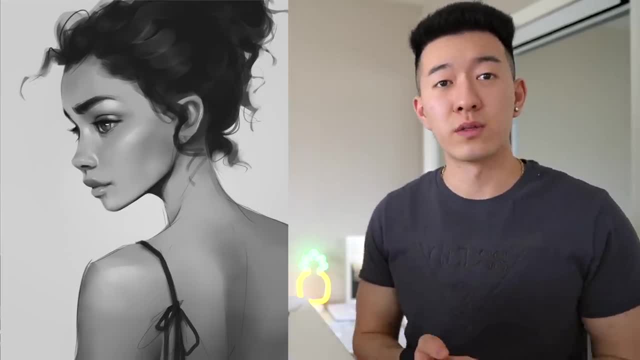 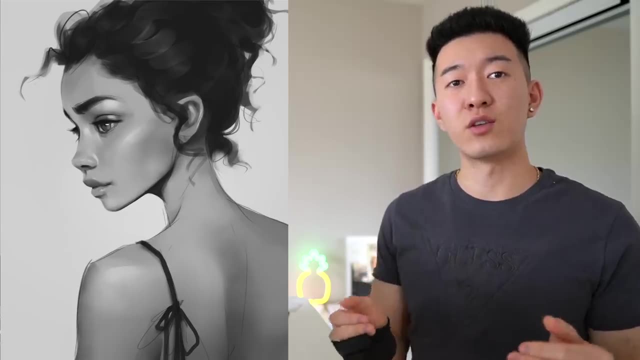 a great way to start practicing because you know, if you go to any kind of an art school, this should be one of the first things that they're going to try to teach you, which is understanding grayscale value and- and this is something that you want to get down before you start moving on to the more 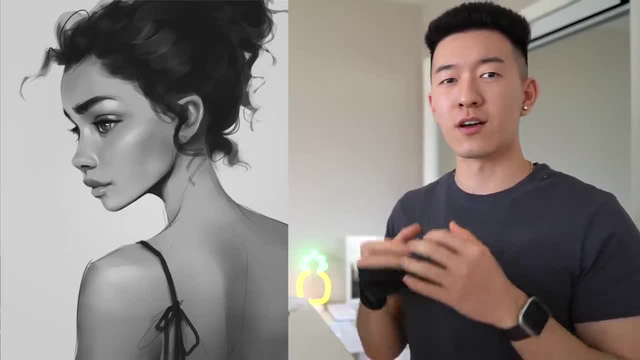 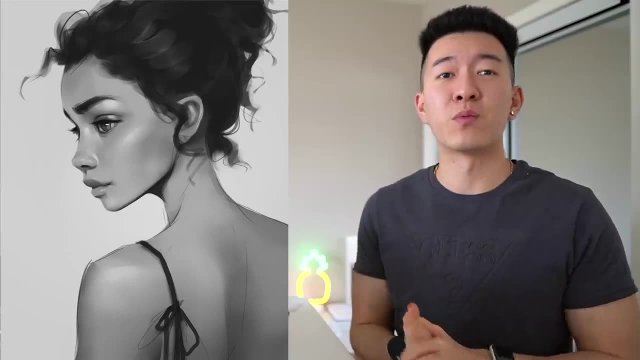 complex stuff like saturation, hue, color theory, all that madness. but yeah, I just wanted to put this video out there because nowadays there's so much information online we don't really know where to start anymore. so you know, if you're a beginner, you're trying to get into a little bit.